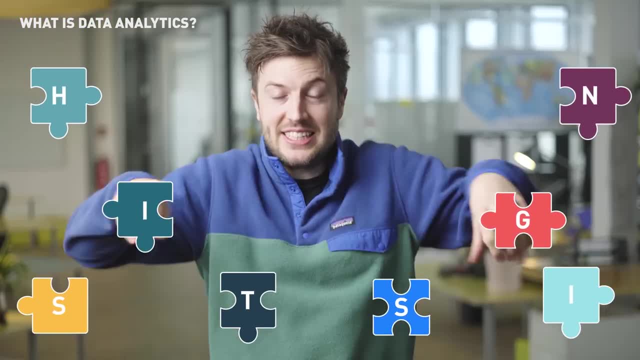 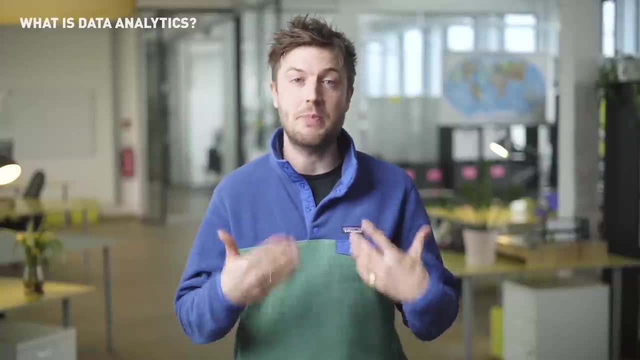 analyst does is they take all this complex jigsaw of data, they take it out and they make it into something which you can really use. Having interpreted the data, the data analyst can then pass these insights on, so that the company can then make the most informed decisions. 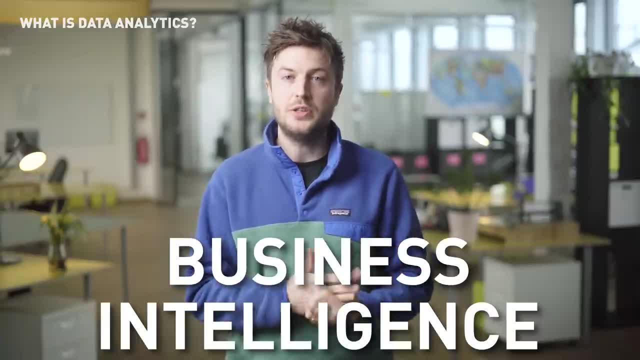 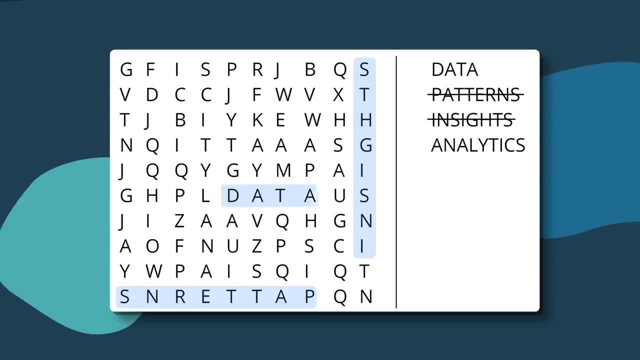 So you can think of data analytics as a kind of business intelligence used to solve problems and challenges that every company has. It's all about finding patterns in the data which can tell you something useful or relevant about the business operations, So, for instance, how customers engage with. 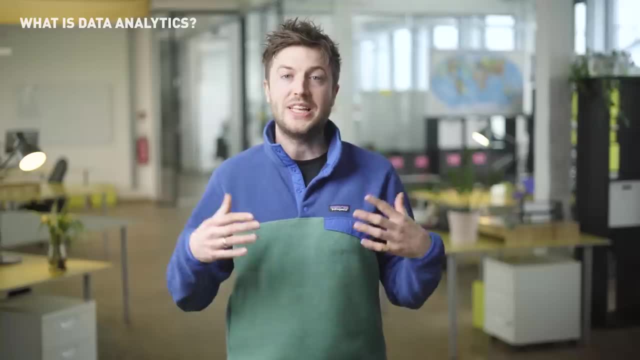 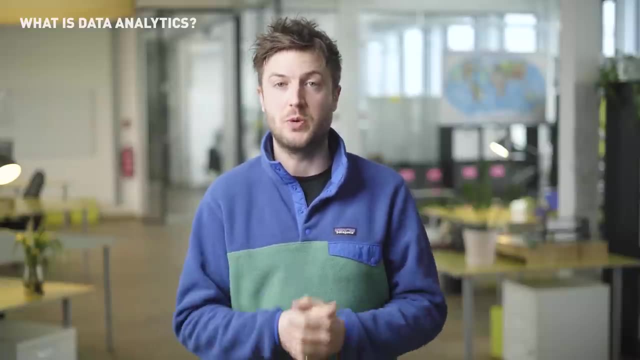 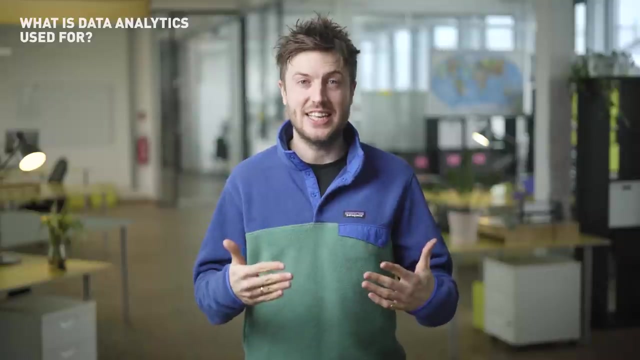 a particular product or employees engage with a particular tool Armed with the insights of data, companies are then able to make better decisions about their audience, company as a whole and the industry in which they work. in Step one, we looked at what data analytics actually is. In step two, we're going to 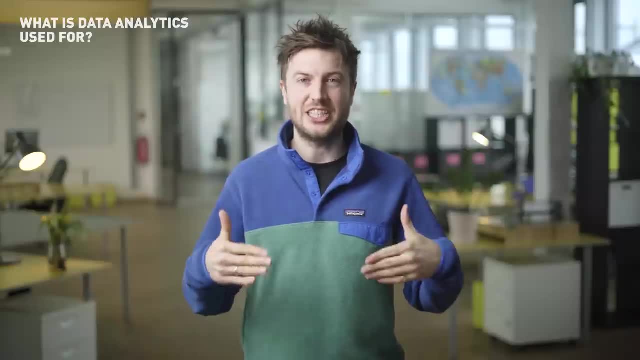 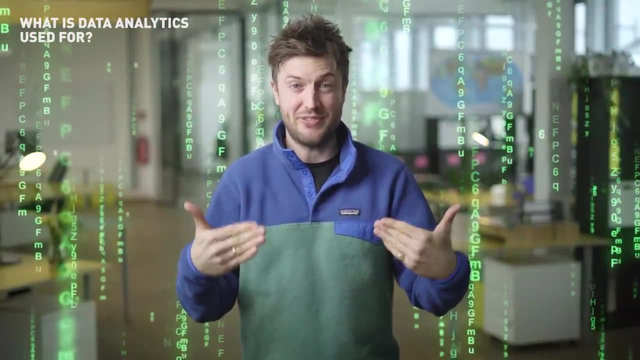 look at how data analytics is used. So what does data analytics actually look like in action and how is it used in the real world? So the fact is, data is everywhere, So it actually has an infinite amount of uses across all kinds of businesses and organisations. 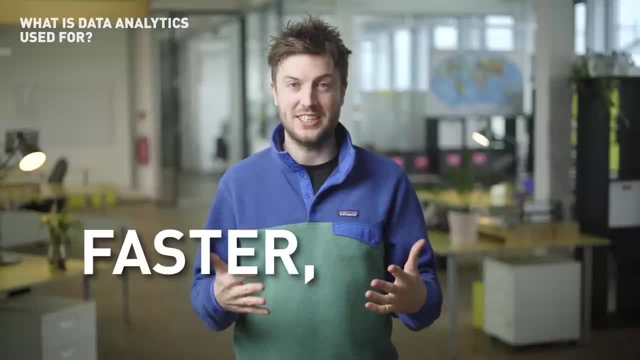 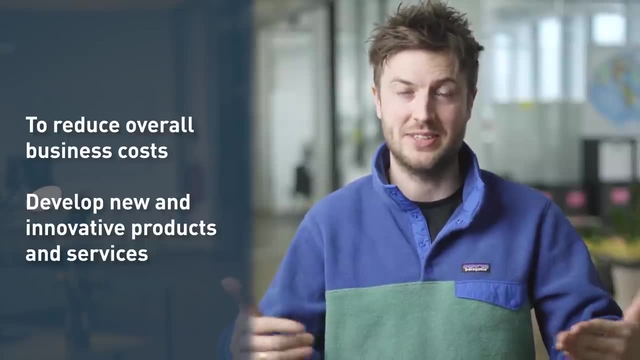 globally. Broadly speaking, data analytics is used to make faster and better business decisions, to reduce overall business costs and to develop new and innovative products and services. In more specific terms, data analytics might be used to do the following: To predict future sales. 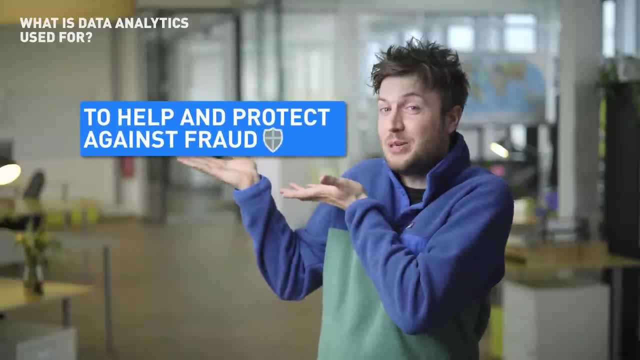 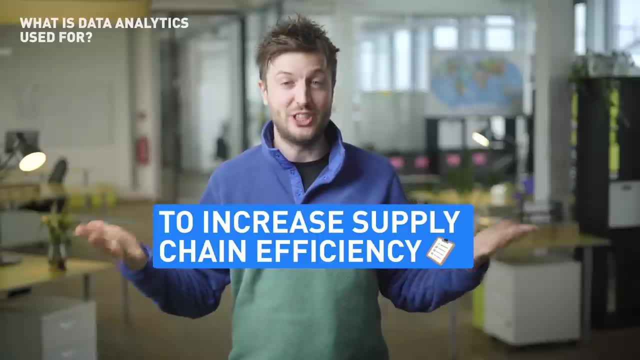 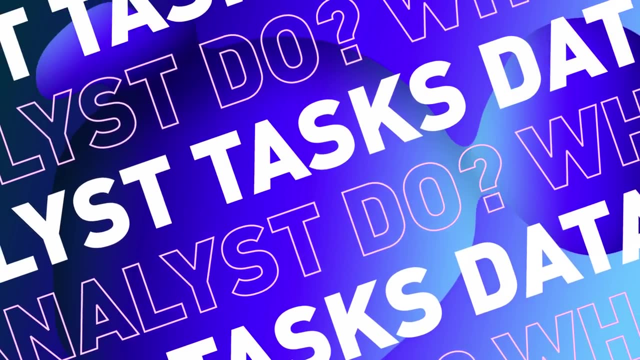 acquisition and retention Or to increase supply chain efficiency. So that gives you a little bit of an overview of what data analytics can be used for in the real world. Step three: let's dive into what a data analyst actually does on a day-to-day basis. 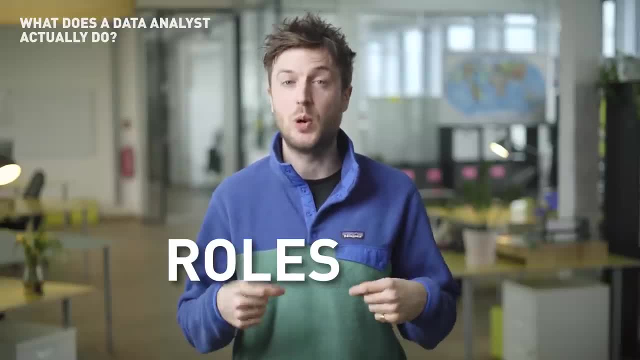 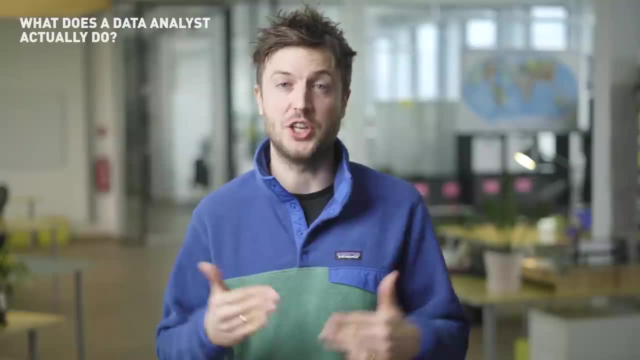 If you're thinking about becoming a data analyst, you're probably interested in the roles and responsibilities that you'll have in the field. Based on some real job ads, here are some typical roles and responsibilities that you'll have to undertake as a data analyst. 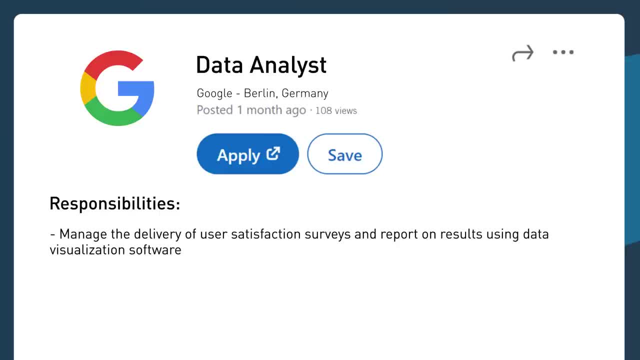 Manage the delivery of user satisfaction surveys and report on results using data visualisation software. Work with business line owners to develop requirements, define success metrics, manage and execute analytical projects and evaluate results. Monitor practices, processes and systems to identify opportunities for improvement. Translate important questions. 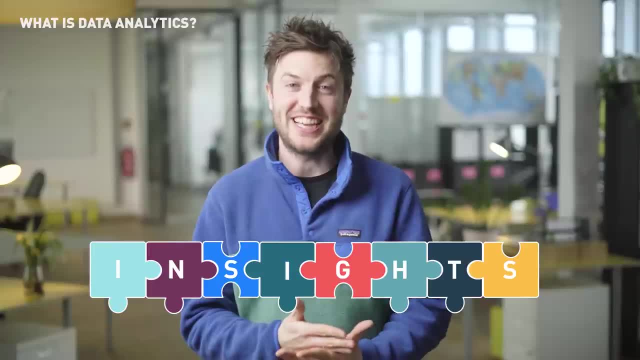 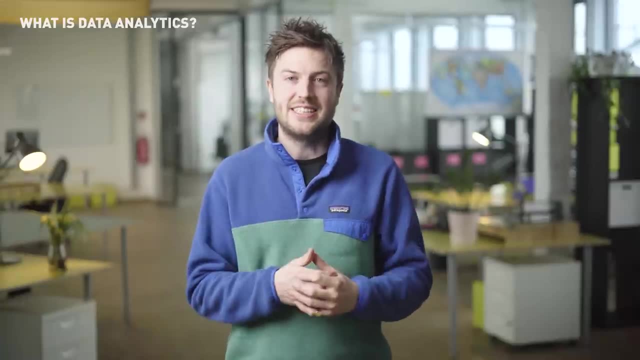 out and they make it into something which you can really use. Having interpreted the data, the data analyst can then pass these insights on so that the company can then make the most informed decisions. So you can think of data analytics as a kind of business intelligence used to solve problems. 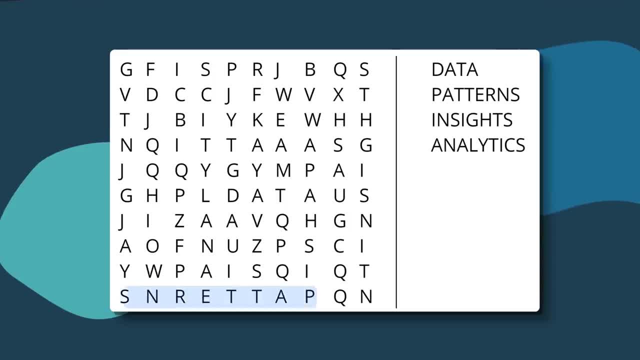 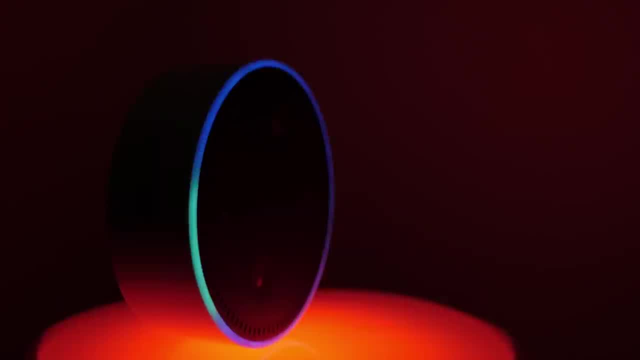 and challenges that every company has. It's all about finding patterns in the data which can tell you something useful or relevant about the business operations, So, for instance, how customers engage with a particular product or employees engage with a particular tool. Armed with the insights of data, companies are then able to make better decisions about. 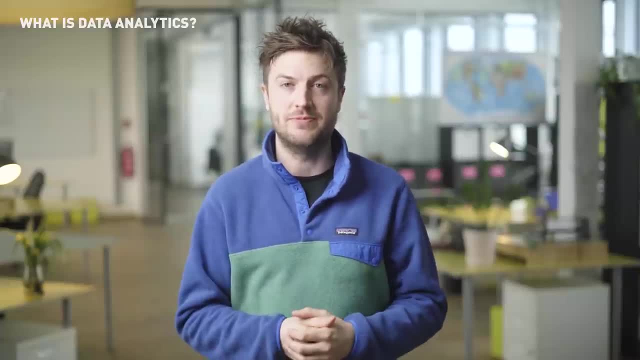 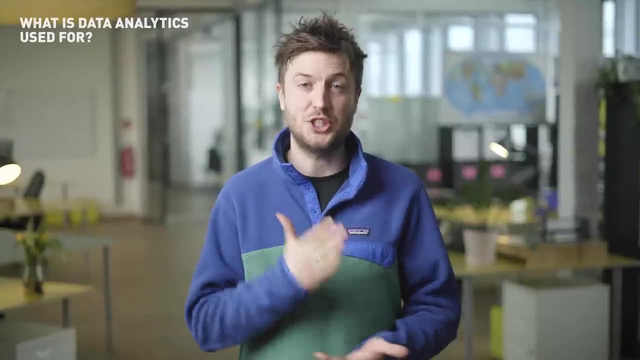 their audience, company as a whole and the industry in which they work. in Step one, we looked at what data analytics actually is. In step two, we're going to look at how data analytics is used. So what does data analytics actually look like? 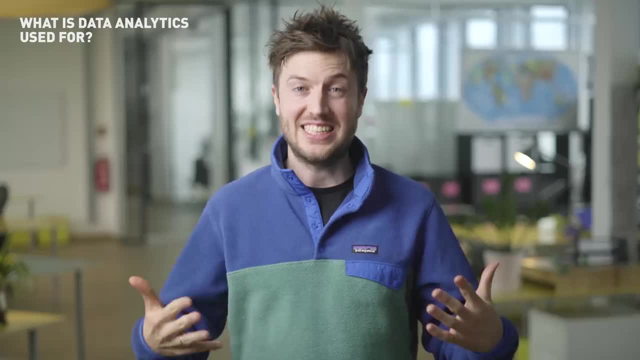 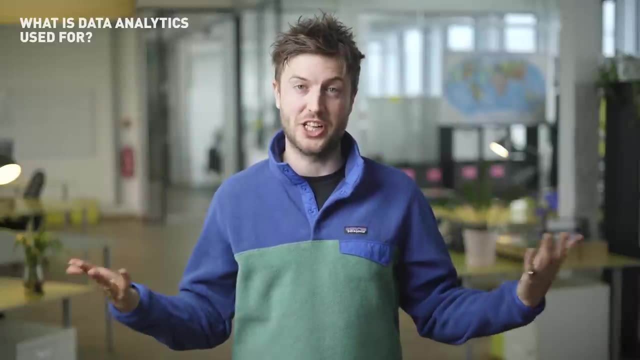 Like in action and how is it used in the real world. So the fact is, data is everywhere, So it actually has an infinite amount of uses across all kinds of businesses and organisations globally. Broadly speaking, data analytics is used to make faster and better business decisions. 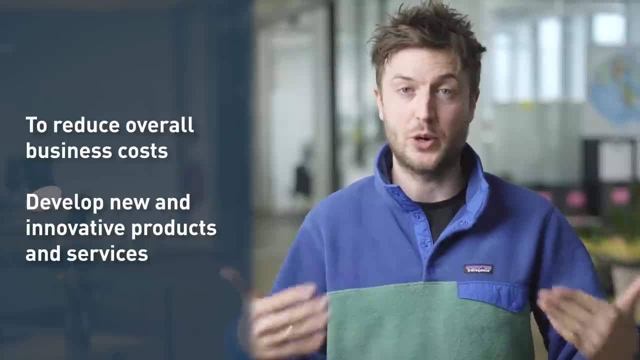 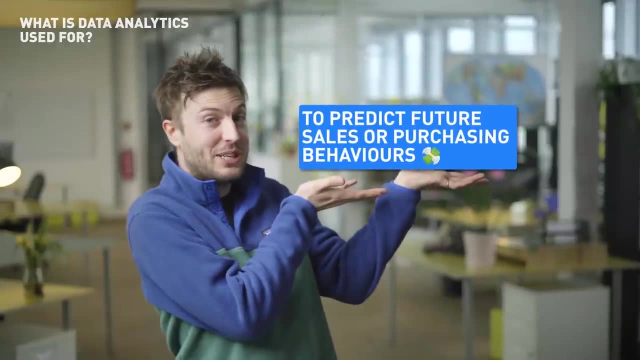 to reduce overall business costs and to develop new and innovative products and services. In more specific terms, data analytics might be used to do the following: To predict future sales or purchasing behaviours. For security purposes. To help and protect it. To protect against fraud. 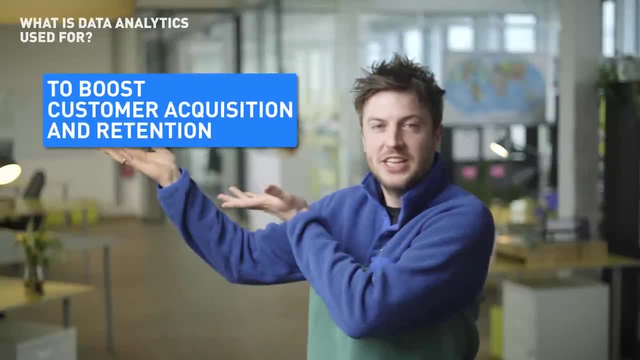 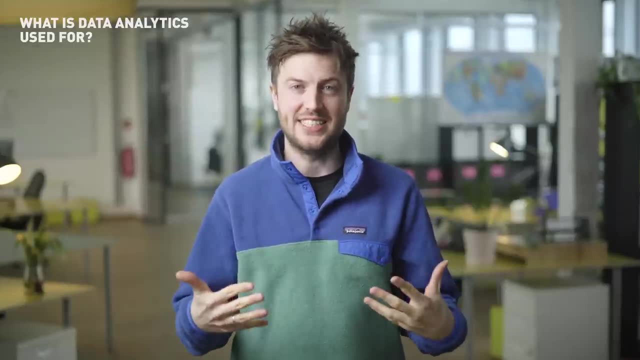 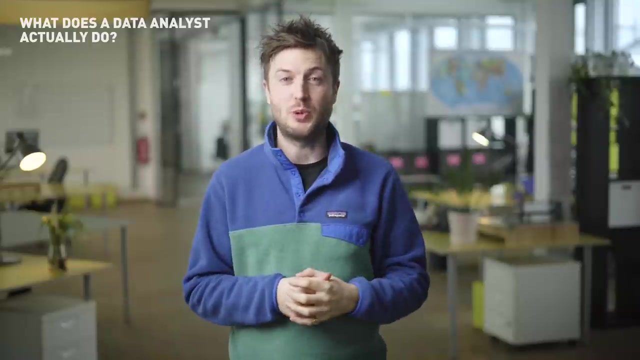 To analyse the effectiveness of marketing campaigns, To boost customer acquisition and retention, Or to increase supply chain efficiency. So that gives you a little bit of an overview of what data analytics can be used for in the real world. Step three: let's dive into what a data analyst actually does on a day to day basis. 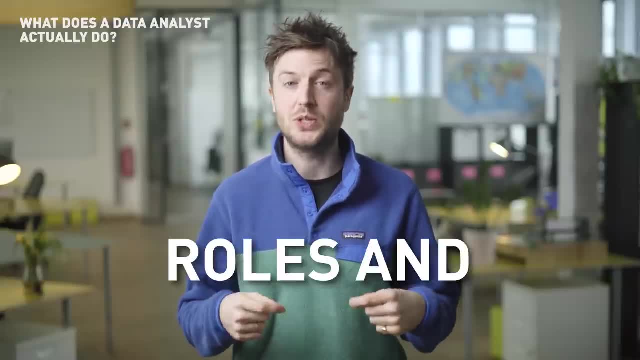 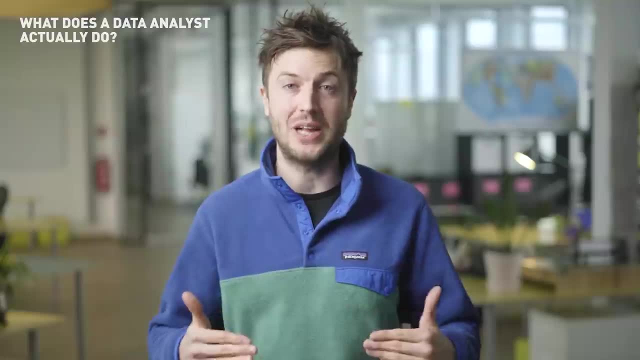 If you're thinking about becoming a data analyst, you're probably interested in the roles and responsibilities that you'll have in the field. Based on some real job ads, Here are some typical roles and responsibilities that you'll have to undertake as a data analyst. 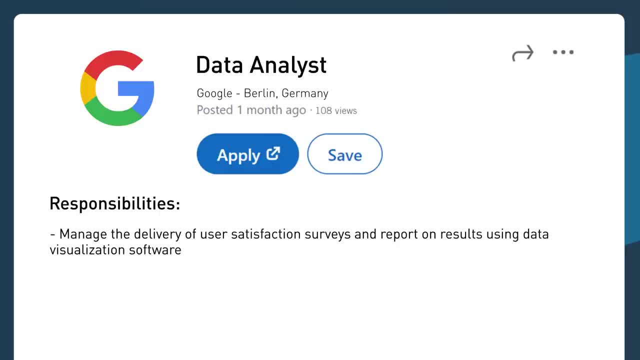 Manage the delivery of user satisfaction surveys and report on results using data visualisation software. Work with business line owners to develop requirements, define success metrics, manage and execute analytical projects and evaluate results. Monitor practices, processes and systems to identify opportunities for improvement. 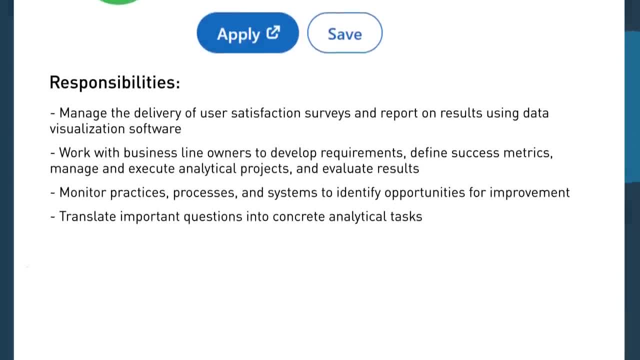 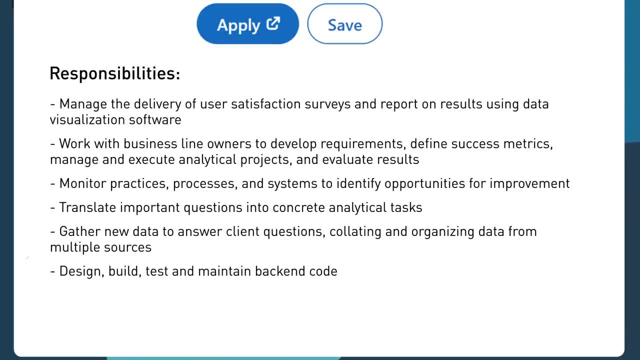 Translate important questions into concrete analytical tasks. gather new data to answer client questions. Collate and organise data from multiple sources. Design, build, test and maintain back-end code. Establish data processes. define data quality criteria and implement data quality processes. Work as part of a team to evaluate and analyse key data that will be used to shape future. 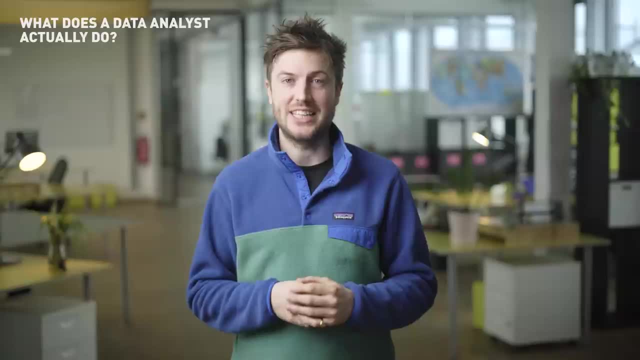 business strategies. So those are just some examples of what a data analyst would be doing in any given role. To learn more about the kinds of things that you'll be undertaking as a data analyst, why not search on job boards like LinkedIn, Indeed and iCrunchdatacom? 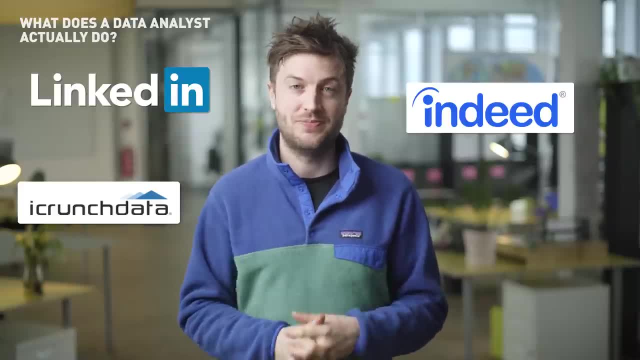 And if you're interested in learning more about the kinds of things that you'll be undertaking as a data analyst, why not search on job boards like LinkedIn, Indeed and iCrunchdatacom? So that's it for today. If you've enjoyed this video, please subscribe to our channel and hit the bell icon to get. 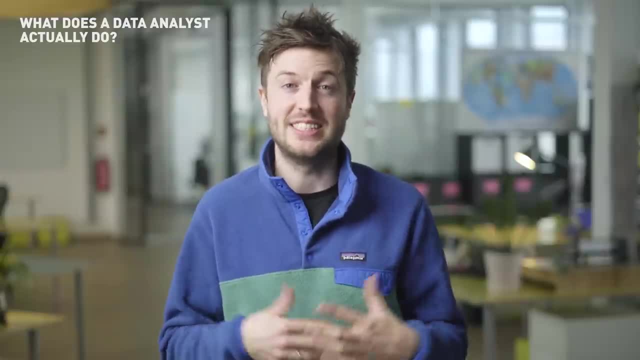 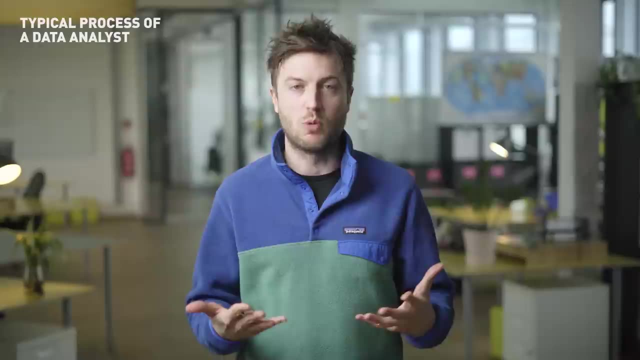 notified about future videos. So that was step three. It was just a broad overview of what you can expect to be doing as a data analyst. So now we've looked at data analytics as a role, we're now going to go into the process. 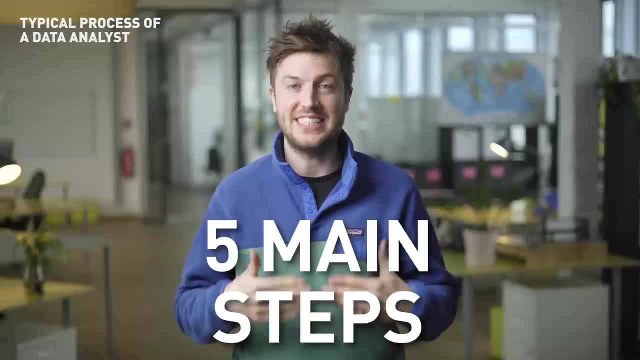 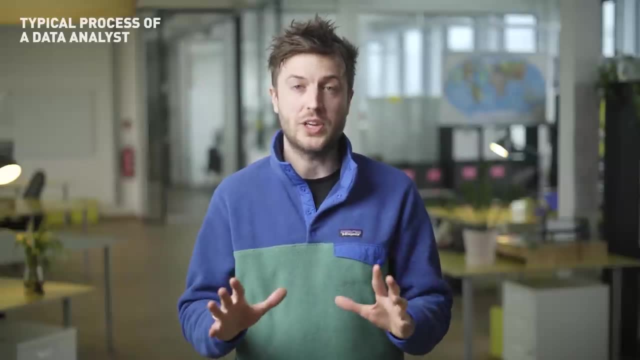 of data analysis. So now we're going to outline the five main steps a data analyst would take when approaching a new project. Step one: define the questions that you want to answer. You need to answer why you're conducting this analysis and what questions and answers you. 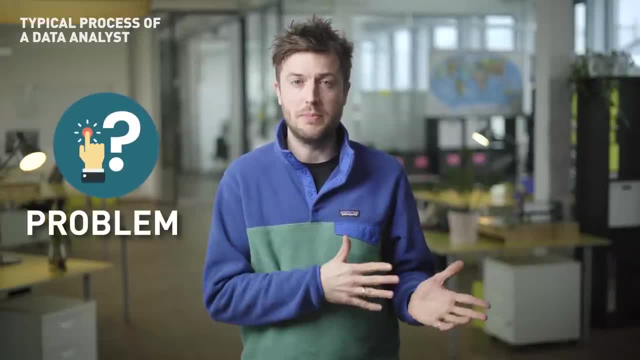 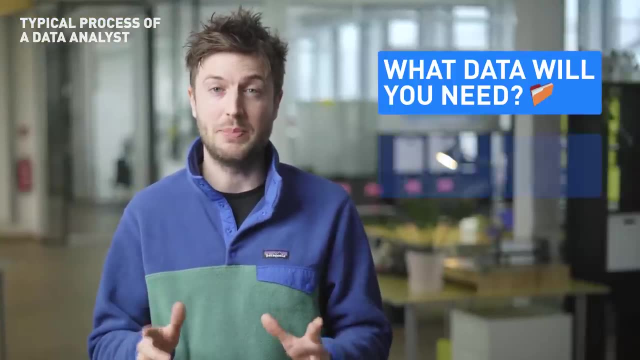 need to find. At this stage, you'll take a clearly defined look at the data analysis and the processes that you need to find, And then you'll make a hypothesis or research question that you can go on and answer. You'll then need to identify what types of data you'll need but, importantly, where it. 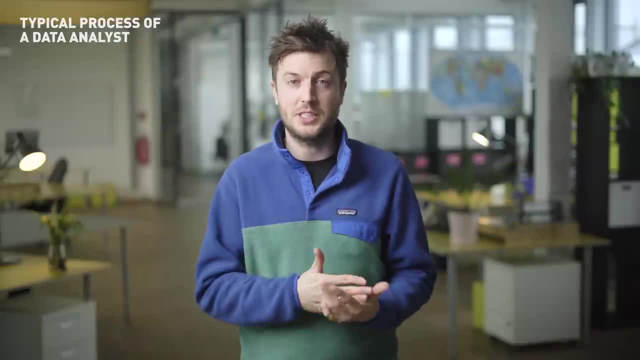 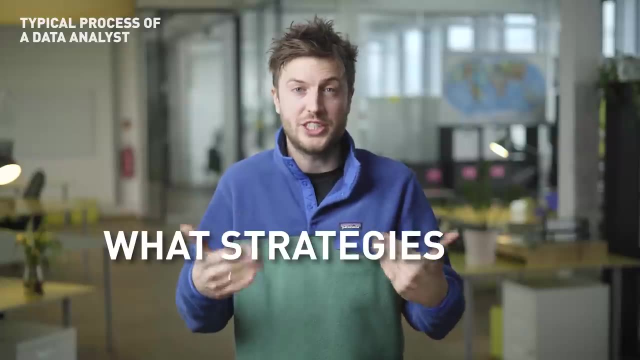 will come from. For instance, a business problem might be that customers aren't subscribing to a paid membership once that free trial ends. Your key question can then be: what kind of strategies can the business implement to retain their customer base? Step two would be to collect this data. 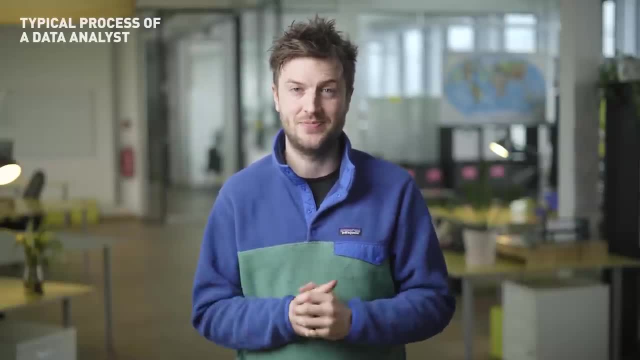 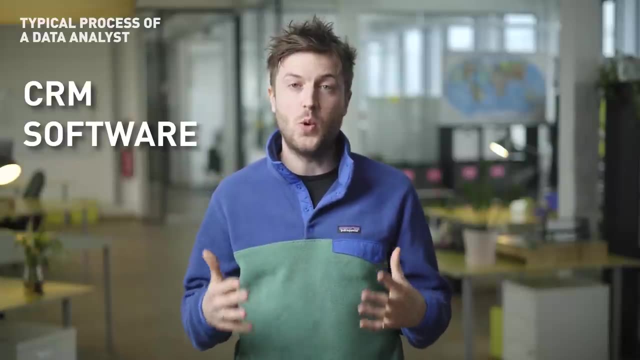 With a clear question in mind: you're ready to start collecting that data? Data analysts will usually go through the process. They'll gather data from primary sources or internal data that the company already has, such as CRM software or email marketing tools. They may turn to secondary or external sources, such as open data sources. 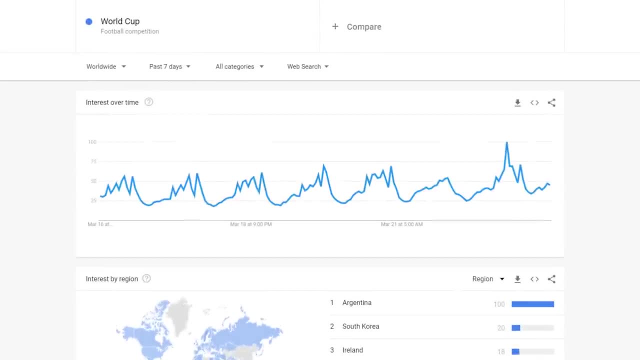 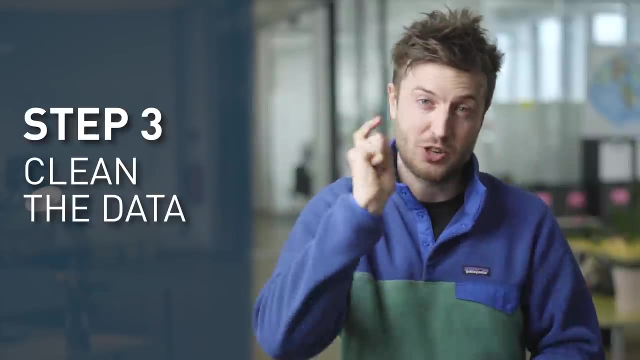 So this can include data from government portals, tools like Google Trends, but also data from international organizations like the World Health Organization. So step three: you need to clean, scrub that data. Once you've got that data, you need to prepare it and ready it for analysis. 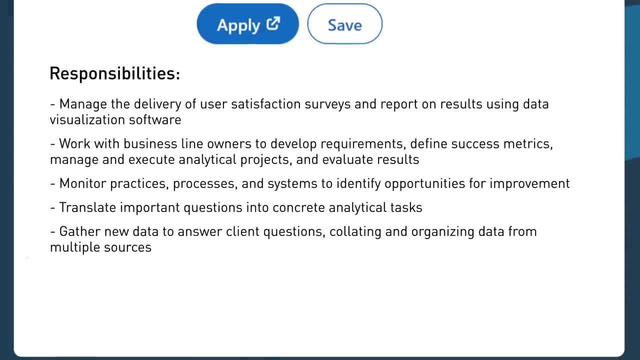 into concrete analytical tasks. Gather new data to answer client questions. collating and organising data from multiple sources. Design, build, test and maintain back-end code. Establish data processes. define data quality criteria and implement data quality processes. Work as part of a team to 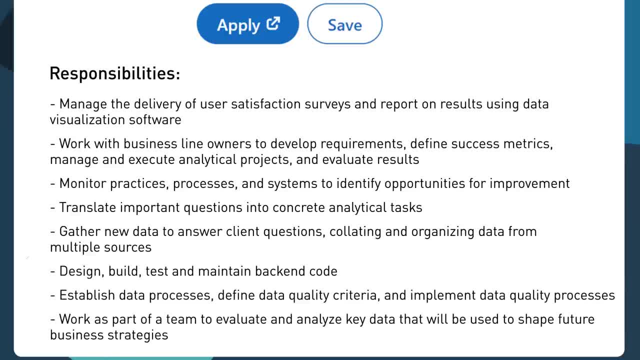 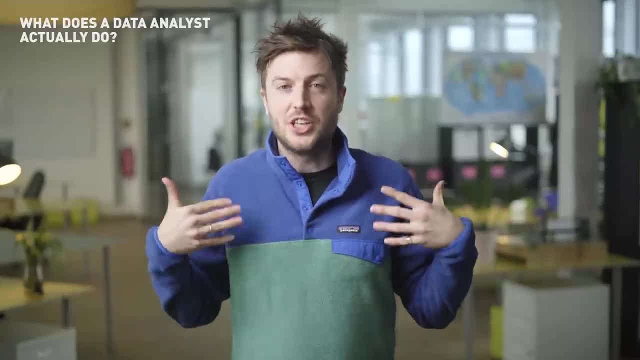 evaluate and analyse key data that will be used to shape future business strategies. So those are just some examples of what a data analyst would be doing in any given role. To learn more about the kinds of things that you'll be undertaking as a data analyst: 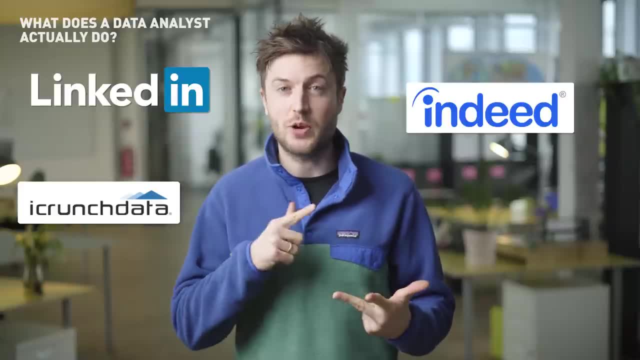 why not search on job boards like LinkedIn, Indeed and icrunchdatacom? So that was step three. Let's dive into your role. So that was step three. Let's dive into your role. Let's dive into your role. Let's dive into your role. 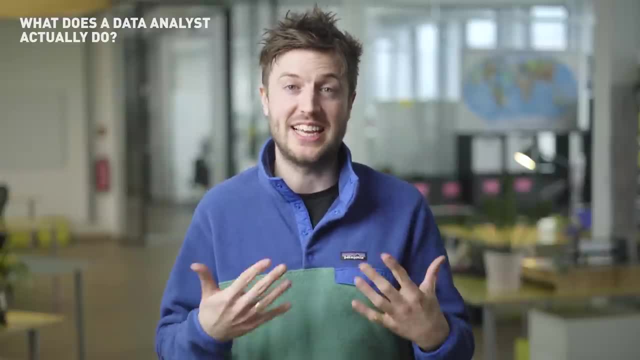 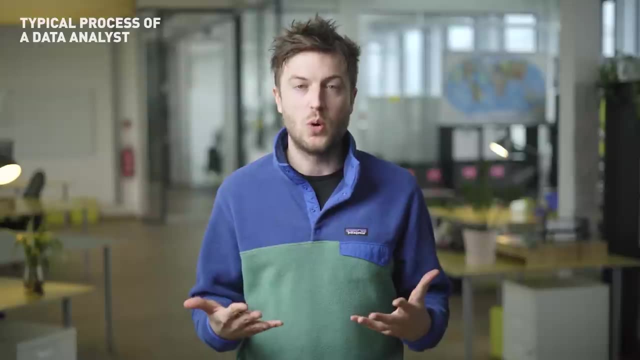 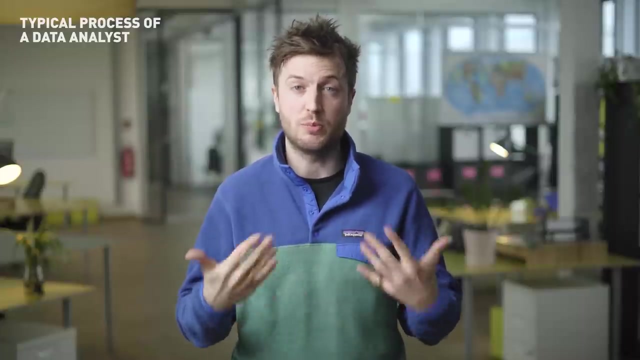 Step three. it was just a broad overview of what you can expect to be doing as a data analyst. So now we've looked at data analytics as a role. we're now going to go into the process of data analysis. So now we're going to outline the five main steps a data analyst would take when approaching a new project. 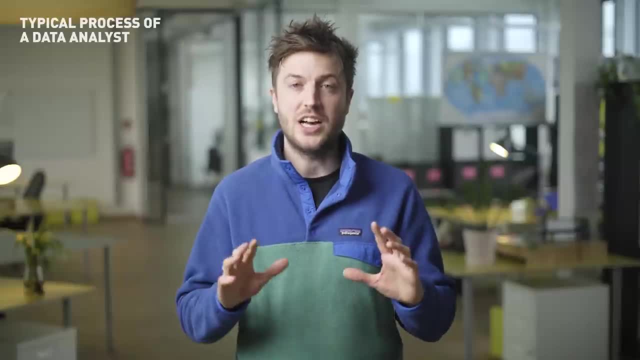 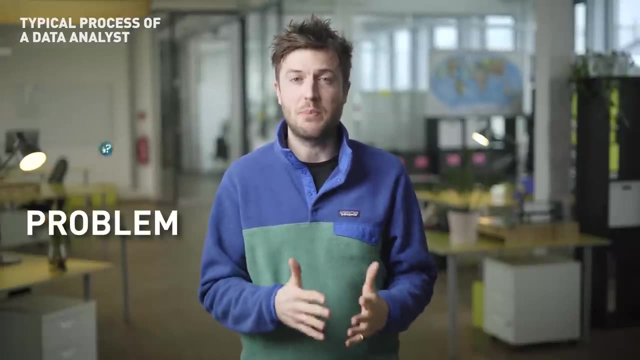 Step one: define the questions that you want to answer. You need to answer why you're conducting this analysis and what questions and answers you need to find. At this stage you'll take a clearly defined problem and then you'll make a hypothesis or research question that you can go on and answer. 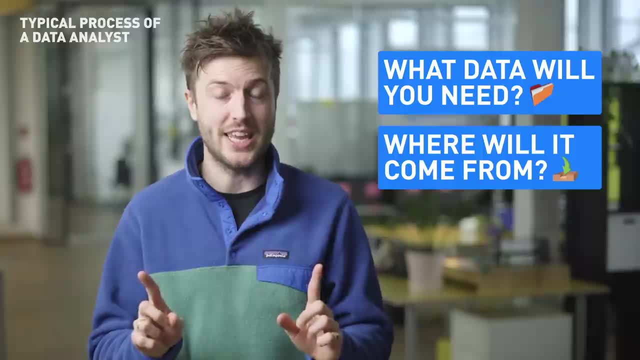 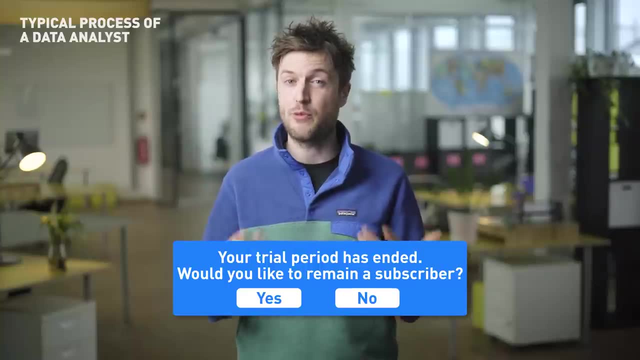 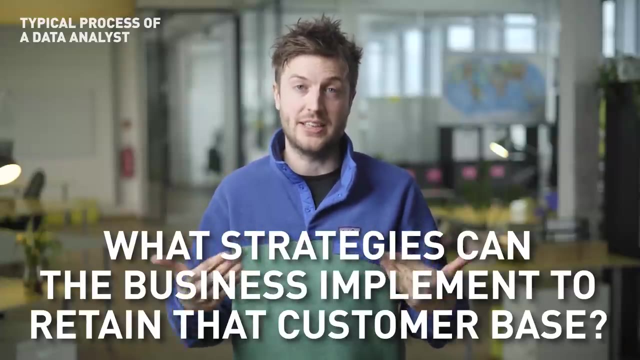 You'll then need to identify what types of data you'll need, but, importantly, where it will come from. For instance, a business problem might be that customers aren't subscribing to a paid membership once that free trial ends. Your key question can then be: what kind of strategies can the business implement to retain their customer base? 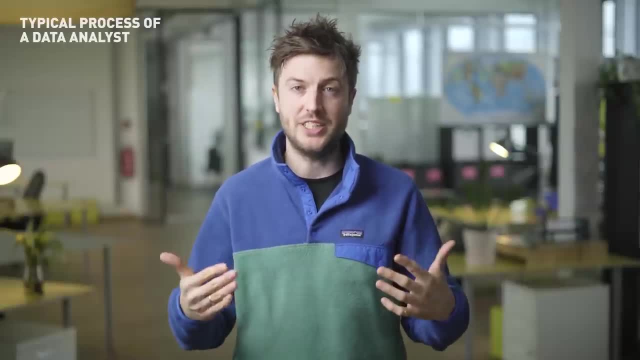 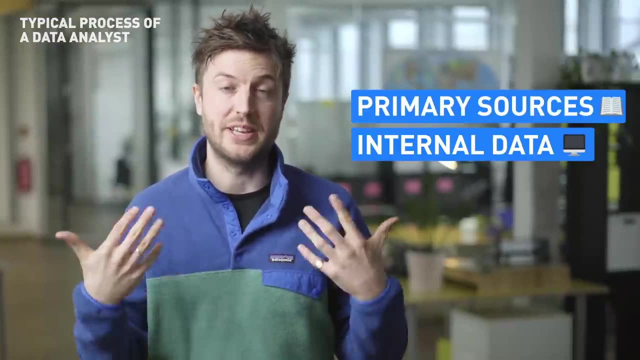 Step two would be to collect this data With a clear question in mind. you're ready to start collecting data, So what are you going to do when you're collecting that data? Data analysts will usually gather data from primary sources or internal data that the company already has, such as CRM software or email marketing tools. 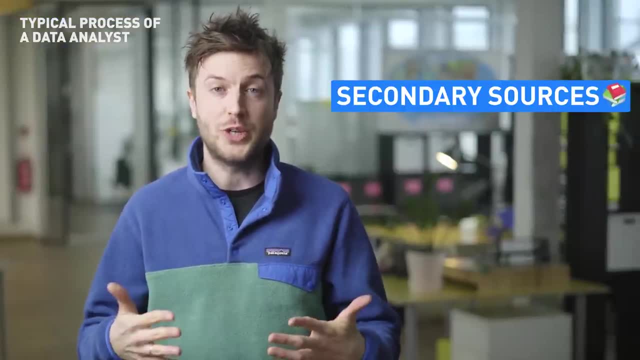 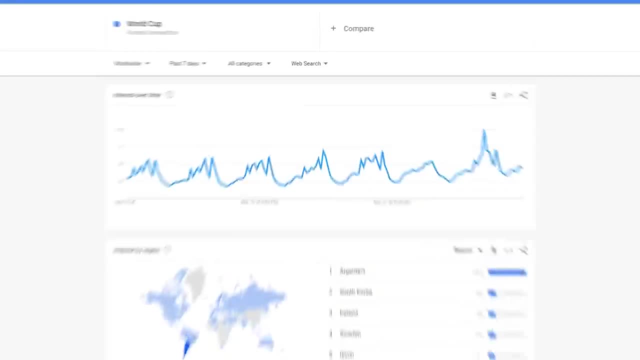 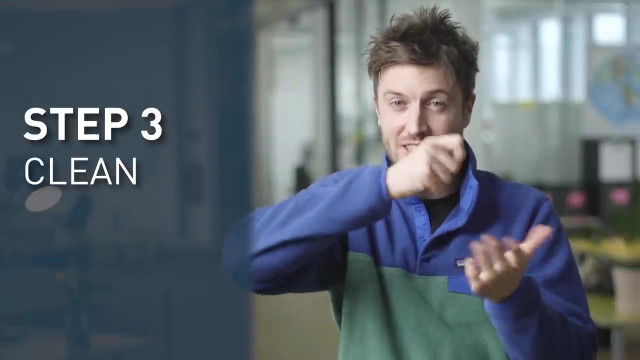 They may tend to secondary or external sources, such as open data sources. So this can include data from government portals, tools like Google Trends, but also data from international organizations like the World Health Organization. So step three: you need to clean. scrub that data. 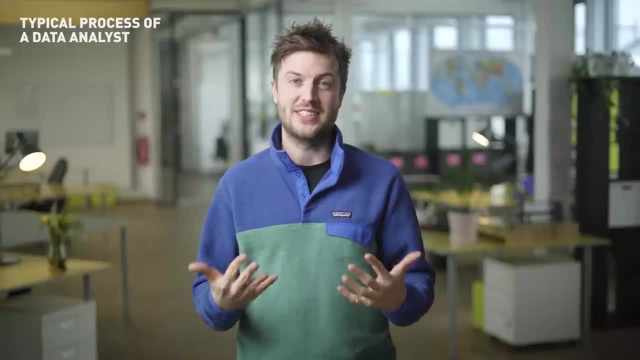 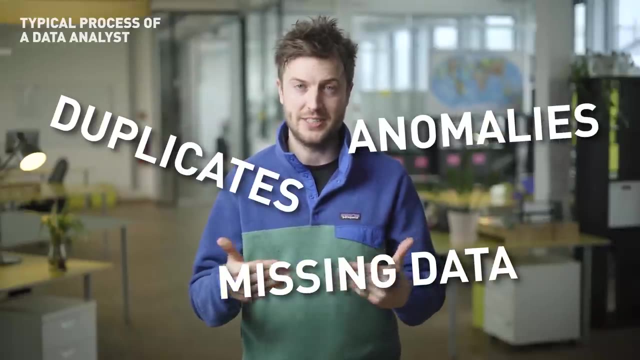 Once you've got that data, you need to prepare it and ready it for analysis. So step three: you need to clean, scrub that data. Once you've got that data, you need to prepare it and ready it for analysis. Your original data might include duplicates, anomalies or missing data which could distort how the data is interpreted. 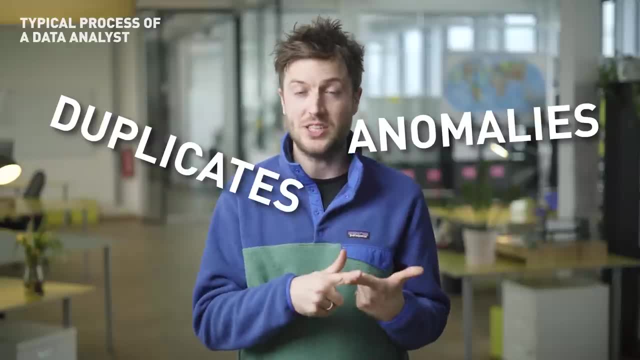 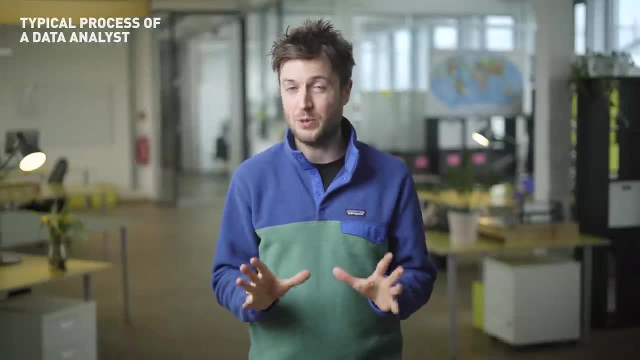 Step three. A lot of data might include duplicates, anomalies or missing data which could distort how the data is interpreted. These all need to be removed. Data cleaning can be a manual task and it can take some time, but it's crucial if you. 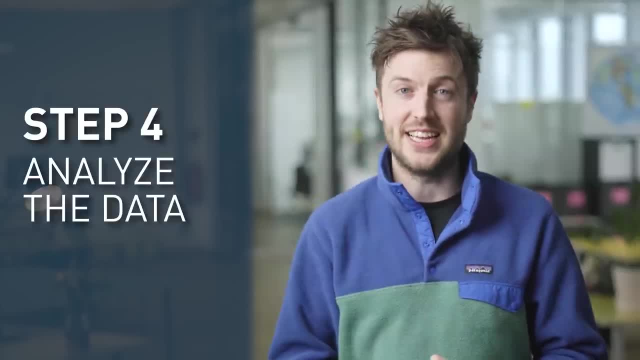 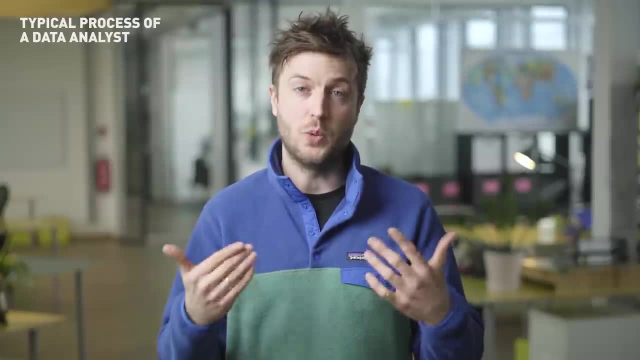 want to get the right business insights. Step four is to analyze the data. Now for the actual analysis. How you analyze the data will depend on the question that you're asking and the kind of data that you're working with, But some common techniques include regression analysis, cluster analysis and time series. 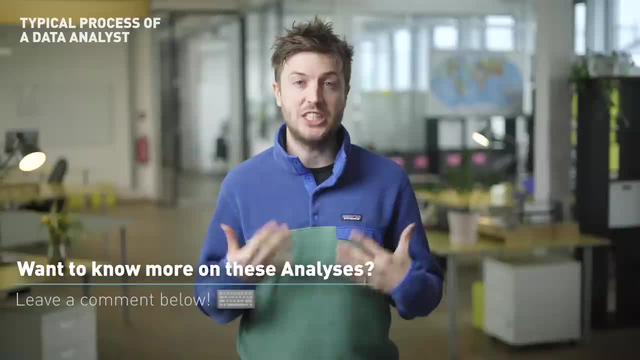 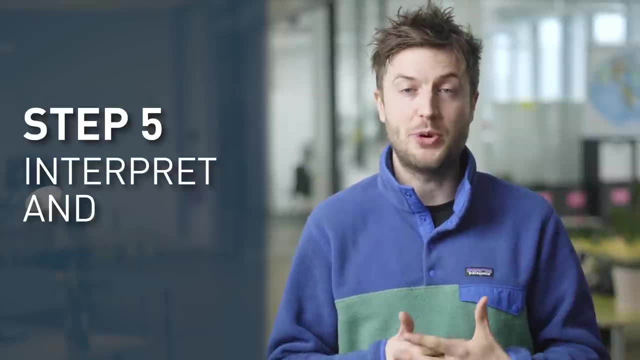 analysis. These are just a few. We're going to go into these analysis terms much deeper in future videos, but if you have any specific questions now, drop us a comment in the comments below. Moving on to step five, we need to interpret and share the results. 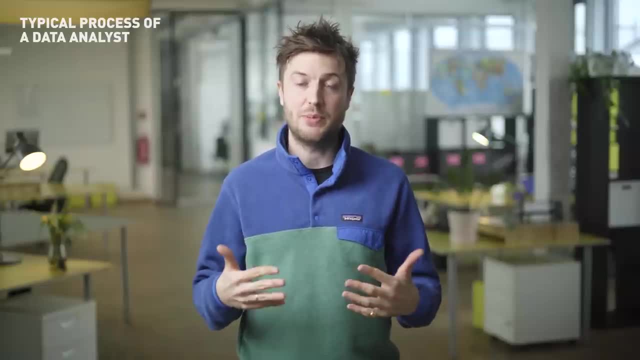 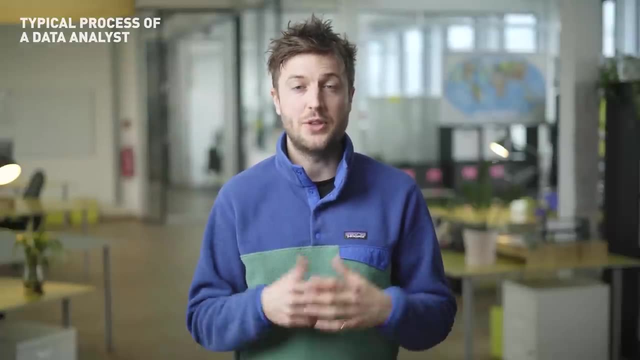 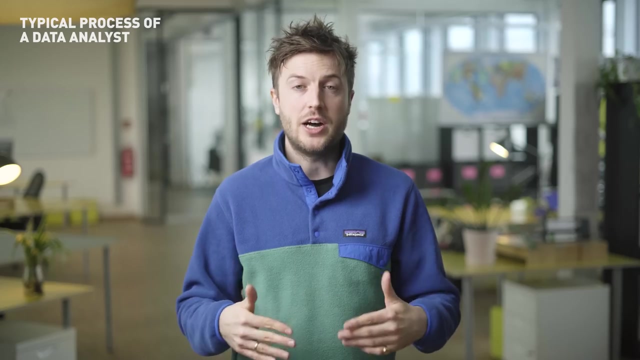 The final step in this process is where data is turned into valuable business insights. Depending on the type of analysis conducted, you'll present your findings in a way that others can understand, In the form of a chart or a graph, for example. At this stage, you'll be able to say what the data analysis actually shows you in regards. 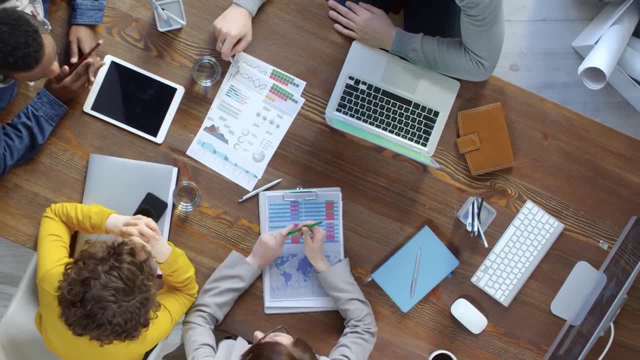 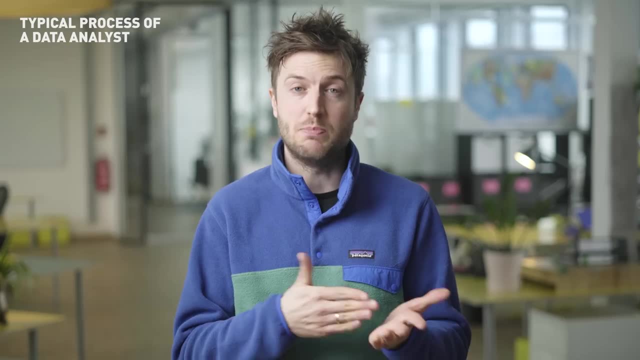 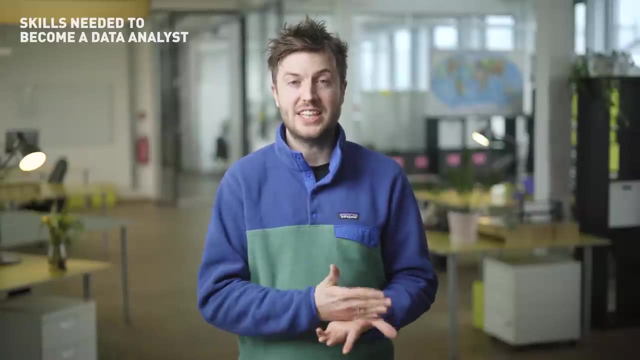 to your initial question or business challenge and you'll collaborate with key stakeholders on how to move forward. This is a great moment to reflect and look at the limitations of your data and what further analysis might be conducted. Rounding off step four, we're going to move on to the next step: what skills you need? 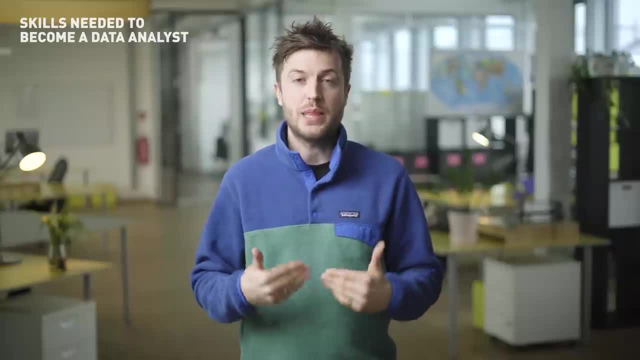 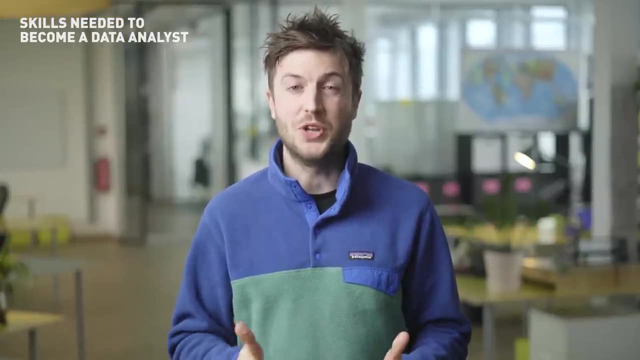 to actually become a data analyst. In addition to the role description and the processes that we've described so far, data analysts are also expected to demonstrate certain skills and abilities. Here are some of the most important half. You'll need to have some hard and soft skills that you'll need to become a data analyst. 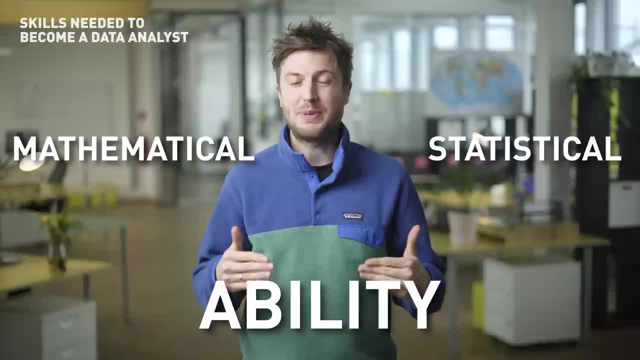 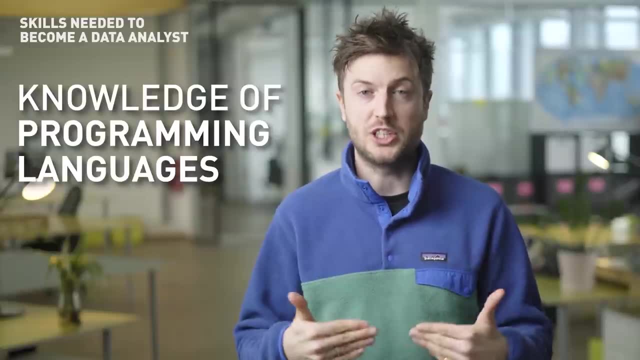 You'll need to have some mathematical and statistical ability. Data analysts spend a lot of their time crunching numbers, so you'll need to have a mathematical brain. You'll have to have some working knowledge of programming languages such as Python, Oracle and SQL. 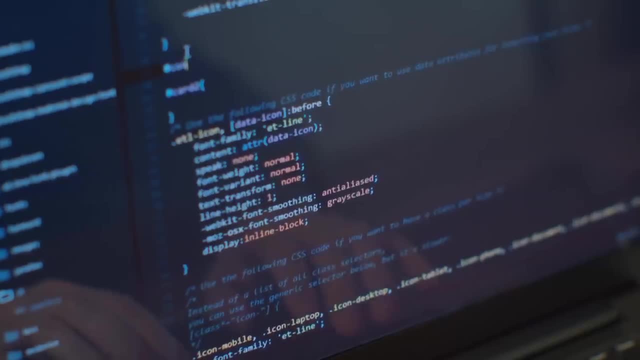 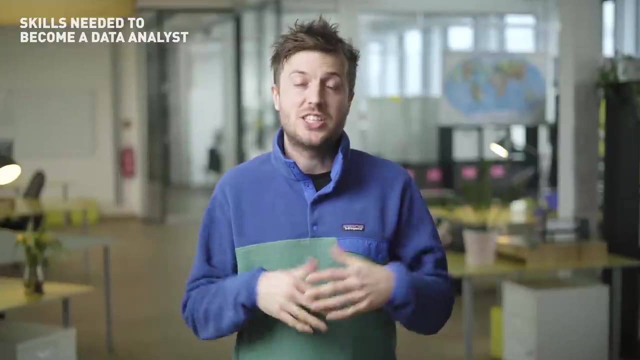 Data analysts rely on a number of programming languages to carry out their work. This may seem daunting at first, but it's nothing that can't be learned over time. with practice, You'll also need an analytical mindset. It's not just about crunching the numbers and sharing your data. 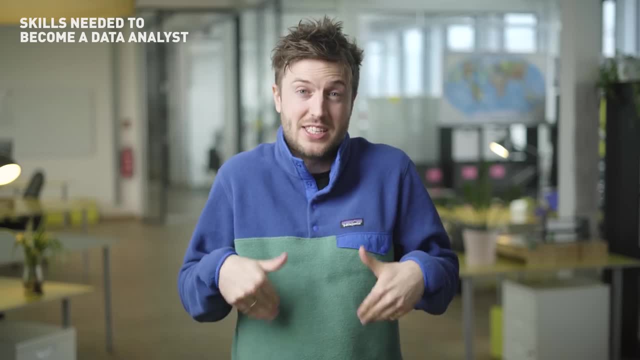 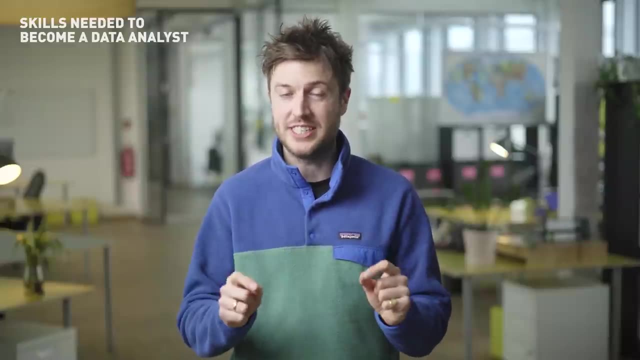 You'll need to have some analytical skills. Sometimes you'll need to dig deeper to understand really what's going on. It's all in the name. An analytical mindset is a must Remember. data analytics is about answering questions and solving business challenges. 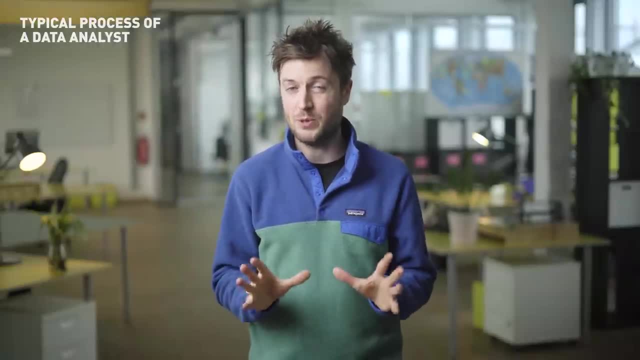 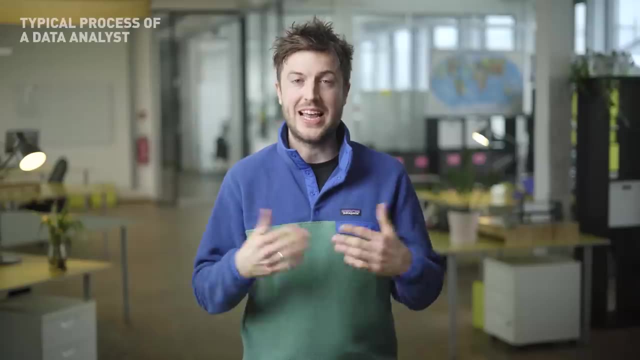 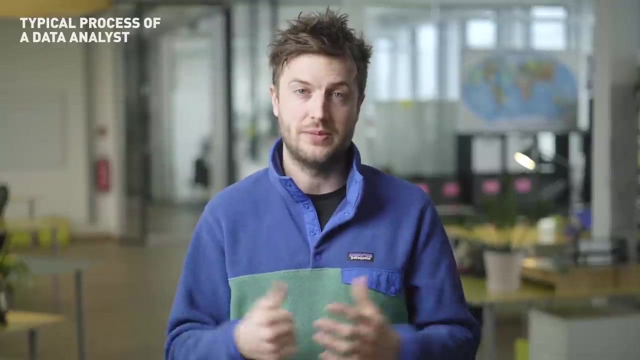 These all need to be removed. Data cleaning can be a manual task and it can take some time, but it's crucial if you want to get the right business insights. Step four is to analyze the data. Now for the actual analysis. How you analyze the data will depend on the question that you're asking and the kind of data that you're working with. 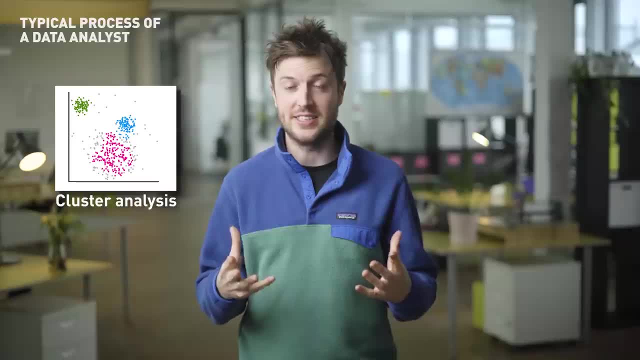 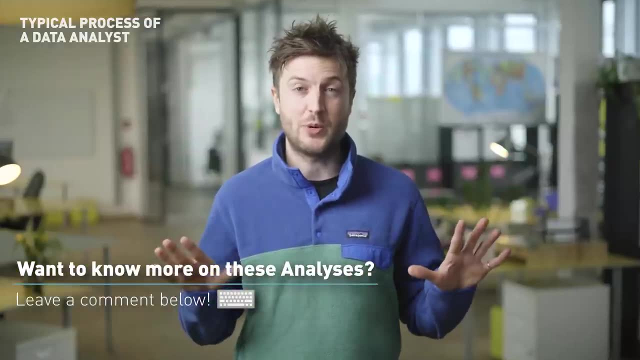 But some common techniques include regression analysis, cluster analysis and time series analysis and time series analysis, to name just a few. We're gonna go into these analysis terms much deeper in future videos, but if you have any specific questions now, drop us a comment in the comments below. 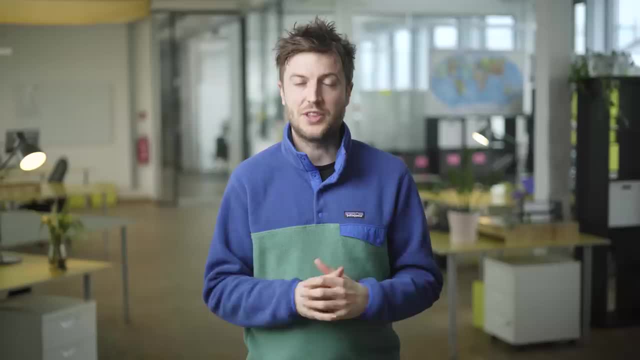 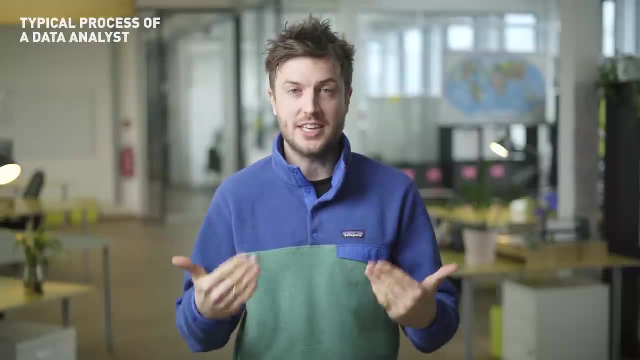 Moving on to step five, we need to interpret and share the results. The final step in this process is where data is turned into valuable business insights. Depending on the type of analysis conducted, you'll present your findings in a way that others can understand. 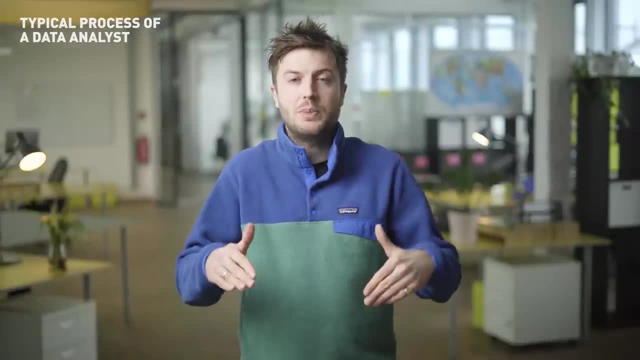 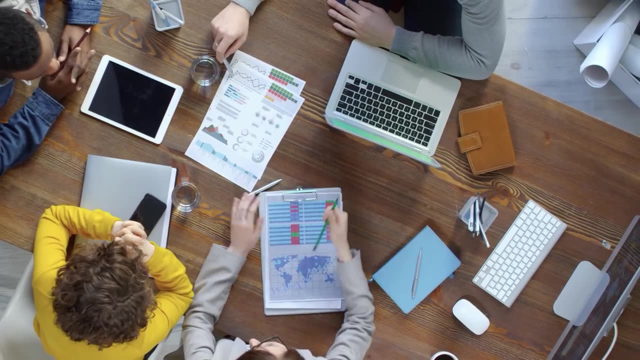 in the form of a chart or a graph, for example. At this stage, you'll be able to say what the data analysis actually shows you in regards to your initial question or business challenge, and you'll collaborate with key stakeholders on how to move forward. 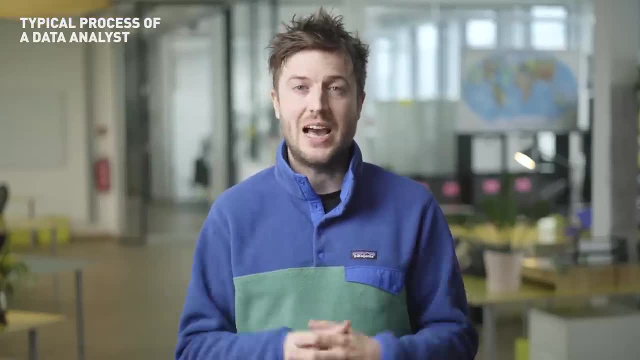 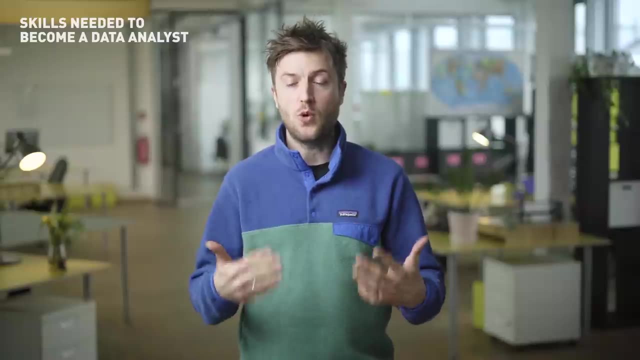 This is a great moment to reflect and look at the limitations of your data and what further analysis might be conducted. Rounding off step four, we're gonna move on to the next step: what skills you need to actually become a data analyst, In addition to the role description. 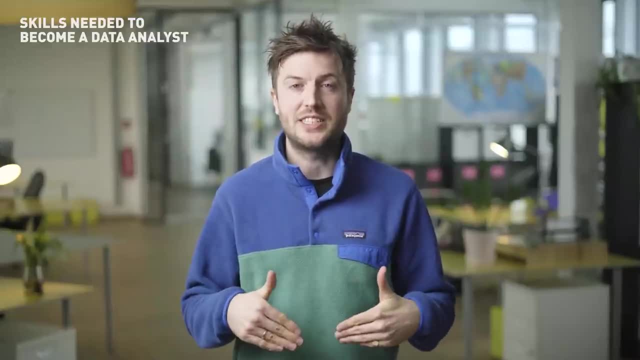 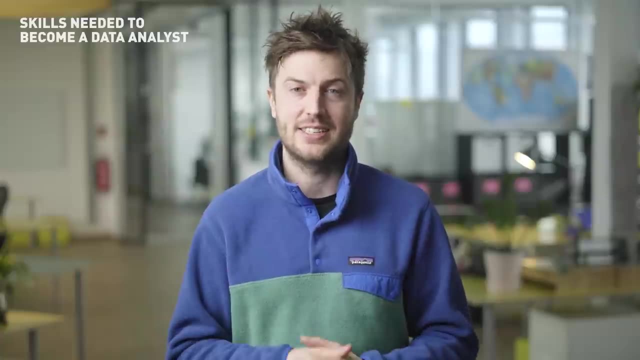 and the processes that we've described so far. data analysts are also expected to demonstrate some of the best and certain skills and abilities. Here are some of the most important hard and soft skills that you'll need to become a data analyst. You'll need to have some mathematical. 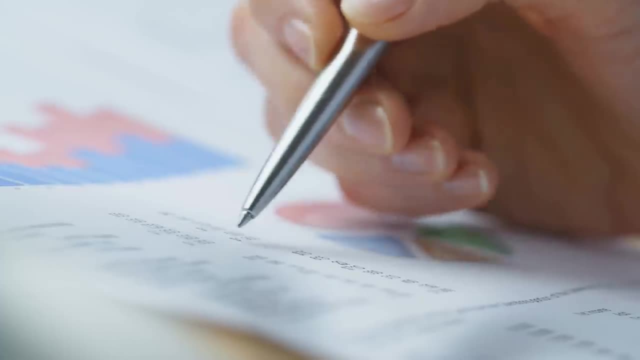 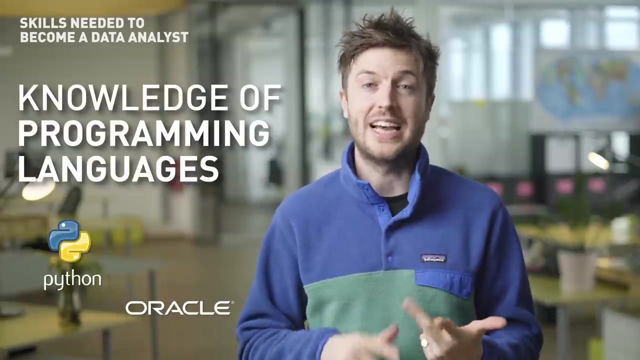 and statistical ability. Data analysts spend a lot of their time crunching numbers, so you'll need to have a mathematical brain. You'll have to have some working knowledge of programming languages such as Python, Oracle and SQL. Data analysts rely on a number of programming languages. 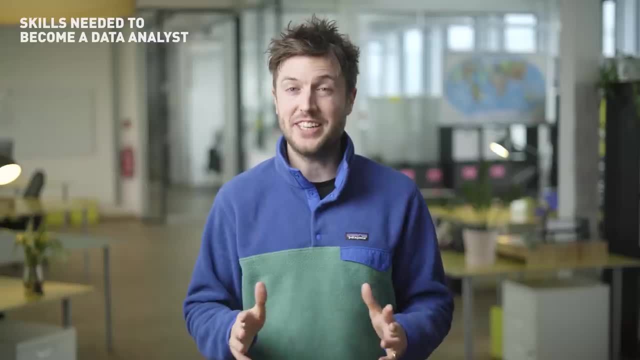 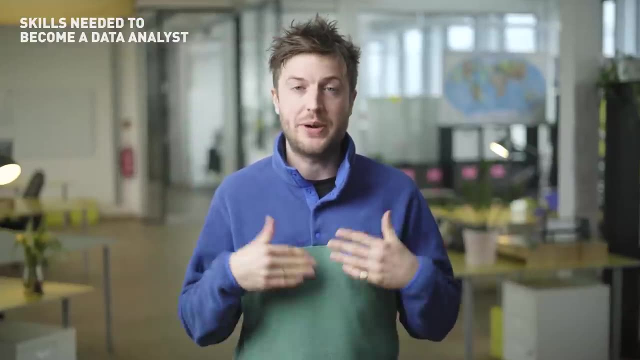 to carry out their work. This may seem daunting at first, but it's nothing that can't be learned over time with practice. You'll also need an analytical mindset. it's not just about crunching the numbers and sharing your data. sometimes you'll need to dig deeper. 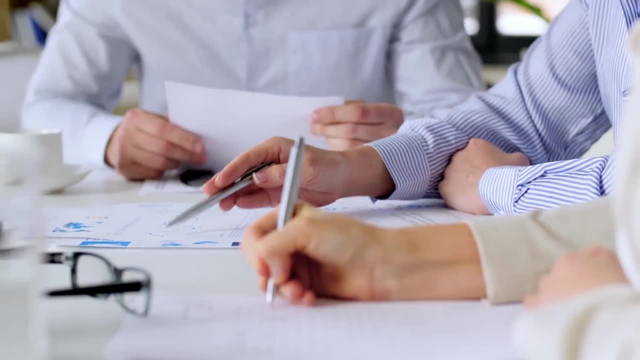 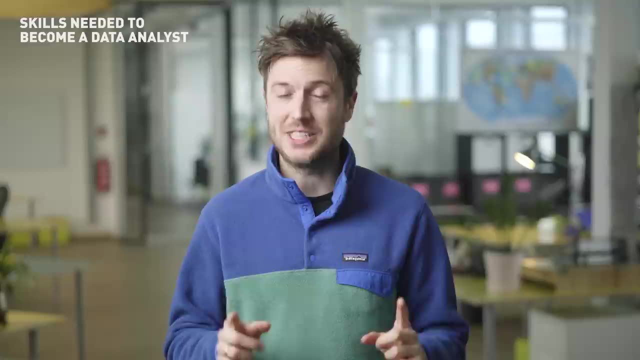 to understand really what's going on. It's all in the name. an analytical mindset is a must Remember. data analytics is about answering questions and solving business challenges, and that requires some keen problem-solving skills. Data analysts have a wide variety of tools.